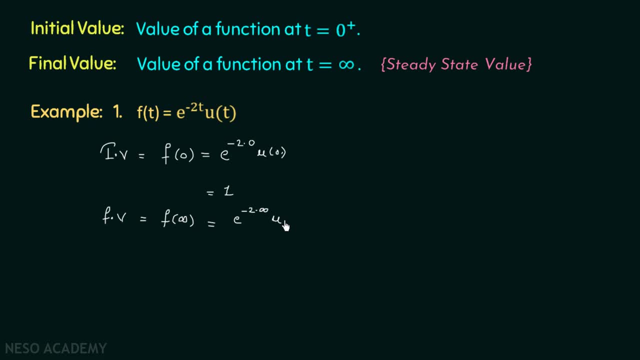 value at t equal to infinity, It will be equal to e to the power minus 2t plus f of infinity. 2 multiplied with infinity. u of infinity. e to the power minus 2 multiplied with infinity is e to the power minus infinity and its value is equal to 0.. So these are the initial and final values for this. 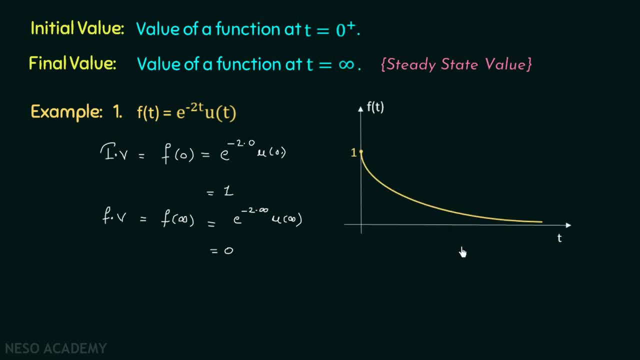 function and if we want to plot this function, then we will have this curve. We can see the initial value, that is, the value at t equal to 0, is equal to 1 and the final value is approaching to 0, at t tending to infinity. So this is an exponentially decaying curve and we can see that it is very easy. 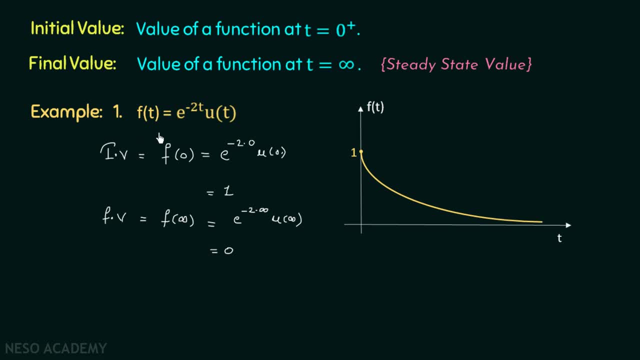 to find out the initial and final values of a function which is in time domain. But suppose if the function is in frequency domain, like f of s equal to 1 over s plus 2, and if we want to find out its initial and final values, then we need to take its inverse Laplace transform to convert this. 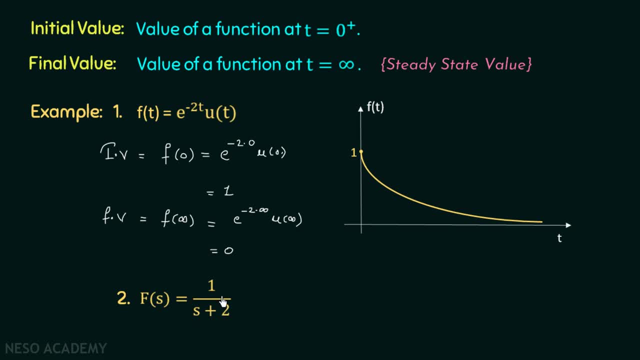 function to its equivalent time domain and then, after that, we will take the values at t equal to 0. And t equal to infinity to find out its initial and final values. But instead of taking the inverse Laplace transform of this function, we will use the initial and final value. theorems Initial and 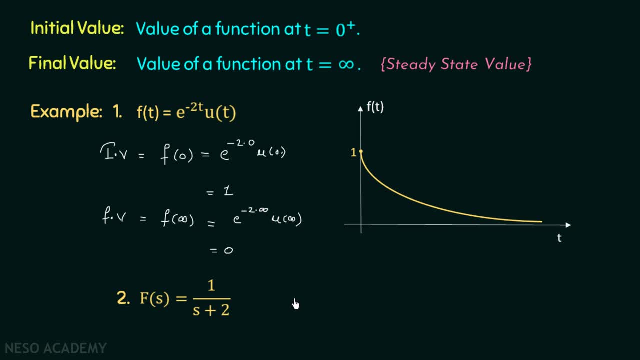 final value theorems are the properties of Laplace transform, by which we can find out the initial and the final values of a function in the s domain. So now we are done with the initial and final value of a function and the significance of initial and final value theorems. We will now discuss 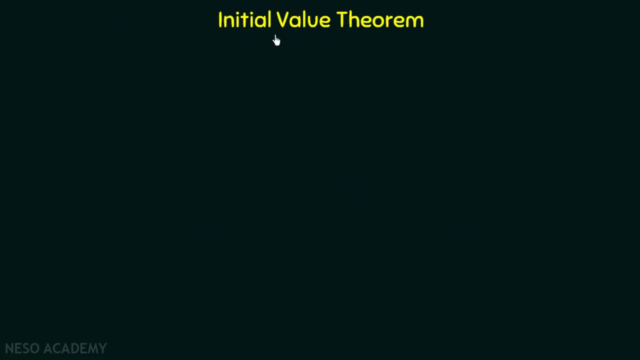 the initial value theorem. The initial value theorem is the property of Laplace transform by which we can find out the initial value of a function in the S domain. Suppose f of t is a time domain function having a Laplace transform f of s, then the initial value of this function. 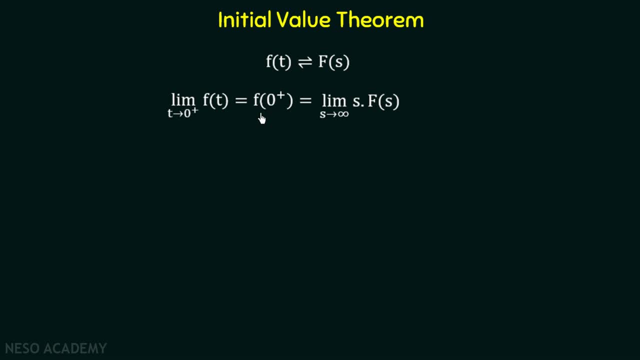 will be limit t tending to 0, f of t, which is equal to f of 0 plus, and it is equal to limit s tending to infinity, s multiplied with f of s, So that the initial vara fermi in this aula is going to be simful. 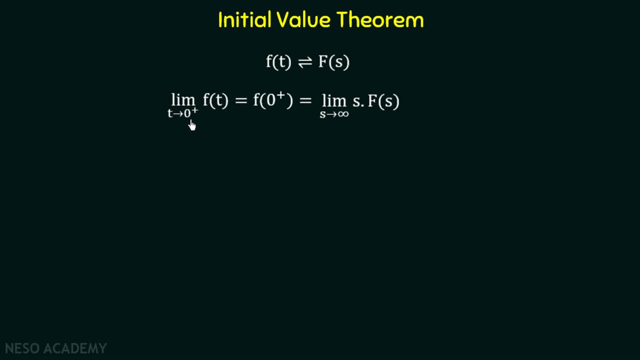 initial value of this function in the time domain is limit. t tending to 0, f of t and its initial value in the s domain is s tending to infinity. s multiplied with f of s. Time and frequency are reciprocal of each other. that's why, in the time domain when t tending to 0 in the s domain s is: 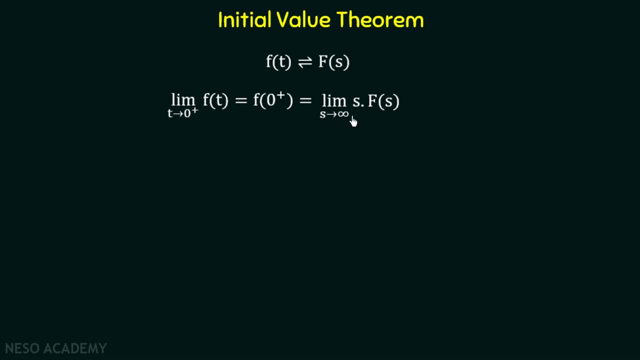 tending to infinity. So both the two are the initial value of the same function. one is in the time domain and the other one is in the frequency domain. So this is the initial value theorem. and now we will understand this theorem with the help of an example. Suppose f of s equal to 1 over s. 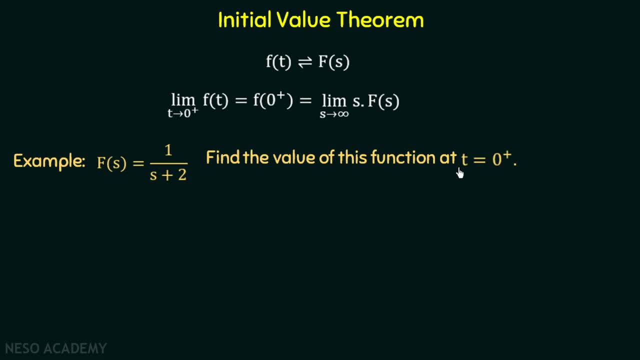 plus 2, find the value of this function at t equal to 0 plus. This is the same function that we have discussed in the earlier section. now we will find out its initial value by the use of initial value theorem. So, moving on to the solution, its initial value in the s domain is limit s tending to. 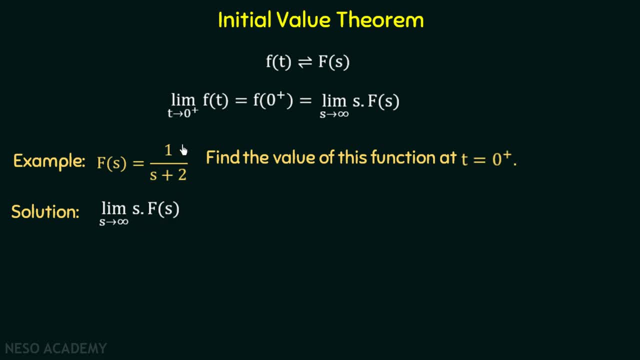 infinity s multiplied with f of s, f of s equal to 1 over s plus 2, so we will have limit s tending to infinity s multiplied with 1 over s plus 2.. Now s is tending to infinity, so we will take s. 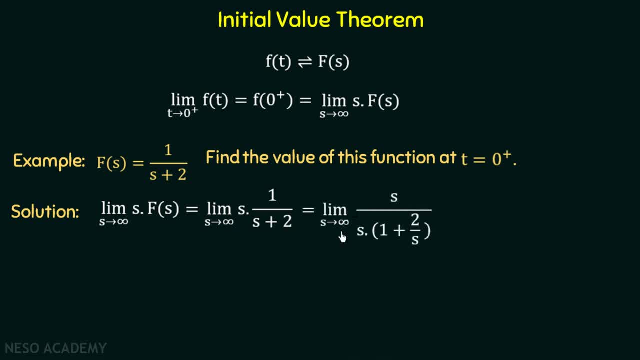 common in the denominator and we will have limit s tending to infinity. s over s multiplied with 1 plus 2 over s We have taken s common in the denominator. Now s in the denominator and in the numerator will get cancelled, And if we take the limit s tending to infinity, then we will have 2. 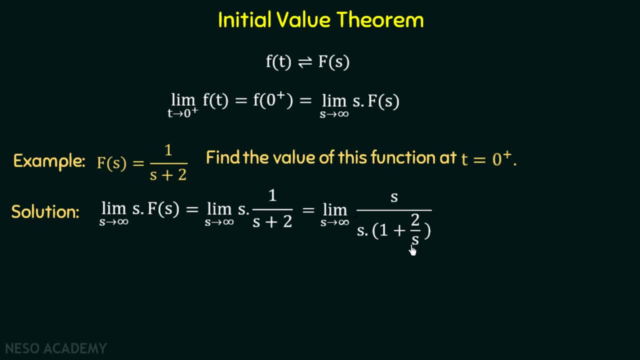 over infinity in this term and it will be equal to 0.. So we will have the limit equal to 1.. So the initial value of this function is equal to 1. And we have calculated this by the use of initial value theorem. So now we are done with the discussion on initial value theorem. we will now discuss the 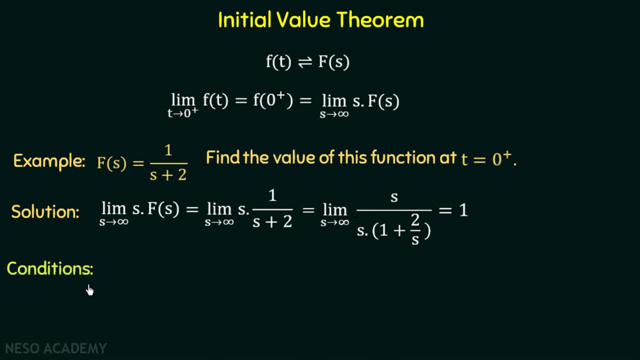 conditions. So for the initial value theorem to be applicable, signal f t must satisfy 2 conditions. Condition number 1 is it is applicable only when f of t is equal to 0, when t is less than 0. That is, from minus infinity to 0, minus the value of the function f of t should be equal. 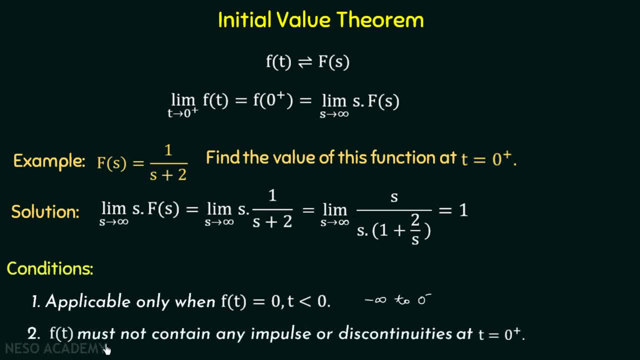 to 0.. The condition number 2 is f of t must not contain any impulse or discontinuities at t equal to 0. So for the initial value theorem to be applicable, signal f t must satisfy 2 conditions. So it should not contain any impulse or any discontinuity at t equal to 0. If these 2 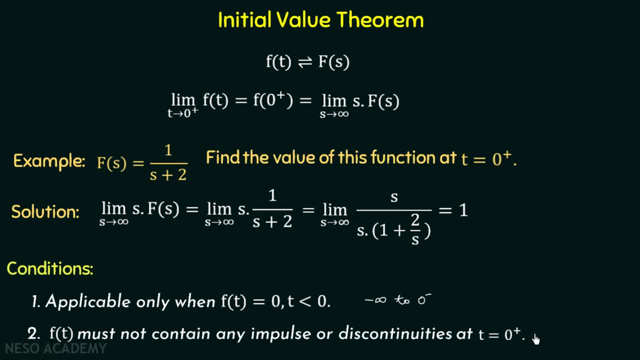 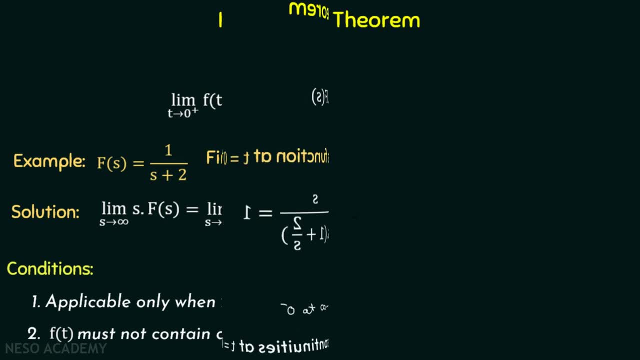 conditions are satisfied, initial value theorem is applicable. And in this way we are done with the discussion on initial value theorem. we will now move on to the final value theorem. The final value theorem is the property of Laplace transform by which we can find out the final value. 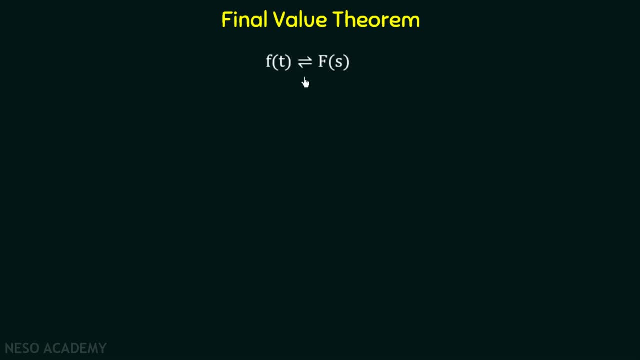 of a function in the s domain. Suppose f of t is having a Laplace transform, f of s, then the final value of a function in the s domain is f of t. So we will now move on to the final value theorem. So the final value of f of t is limit, t tending to infinity, f of t which is equal to f of infinity. 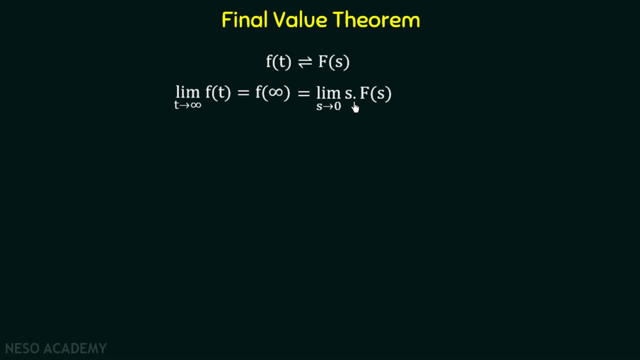 and is equal to limit s tending to 0, s multiplied with f of s. So the final value of this function in the time domain is limit t tending to infinity, f of t, And the final value in the s domain is limit s tending to 0, s multiplied with f of s. So, in the time domain when t is tending to infinity, 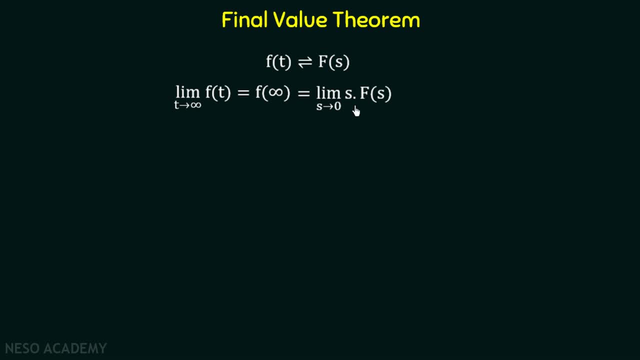 in the s domain, s is tending to 0, s multiplied with f of s, So in the time domain when t is tending to 0.. Both of them are representing the final value of the same function, but one is in. 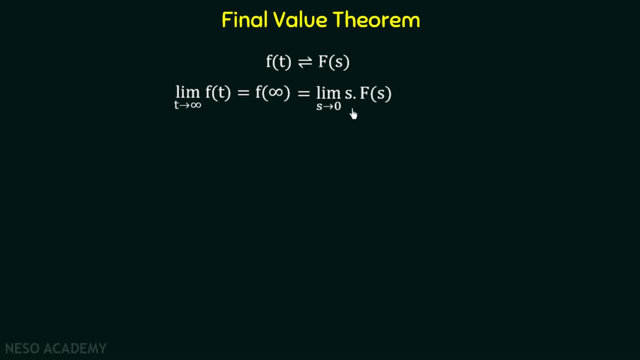 the time domain and the other one is in the frequency domain. So this is the final value theorem and we will understand this theorem with the help of an example. And the example is given as f of s equal to 1 over s plus 2.. Find the value of this function at t equal to infinite. 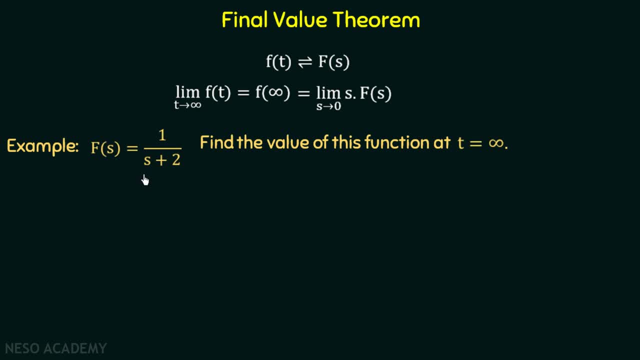 We are having the same example and we will now find out its final value by the use of final value theorem. So, moving on to the solution, the final value of a function is limit t tending to infinity f of t in the time domain. So limit t tending to infinity f of t, which is the final. 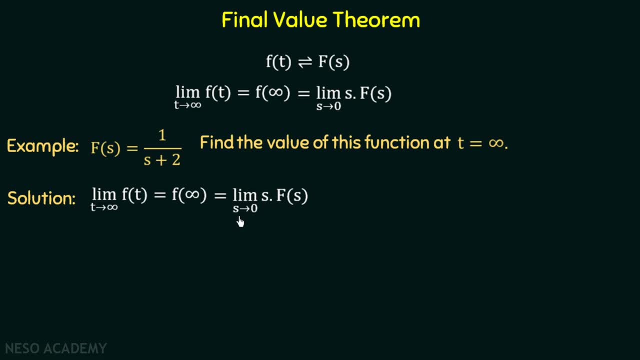 value and in the s domain it is equal to limit s tending to 0 s multiplied with f of s, and f of s is equal to 1 over s plus 2.. So we will have limit s tending to 0 s multiplied with 1 over s plus 2.. 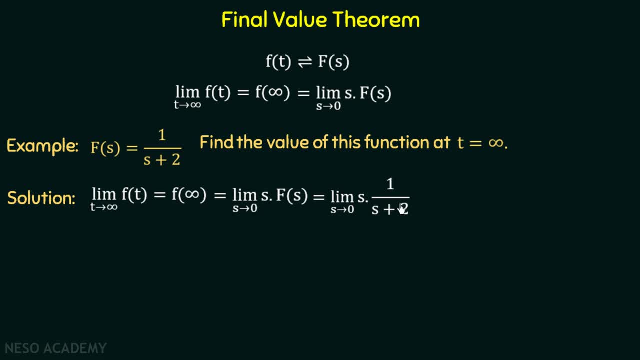 Now, if we substitute the value of limit s tending to 0 here, we will get the value of limit equal to 0. So the final value of this function is equal to 0, and we have calculated this by the use of final value theorem. 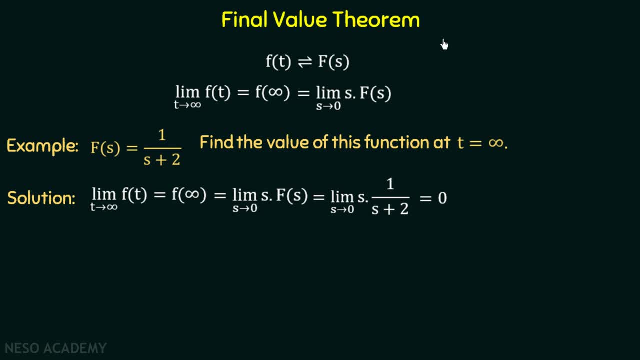 So now we are done with the discussion on final value theorem. We will now move on to the conditions of final value theorem. So for the final value theorem to be applicable, signal f? s must satisfy two conditions. Condition number one is: all the poles of f? s must lie in the left half. 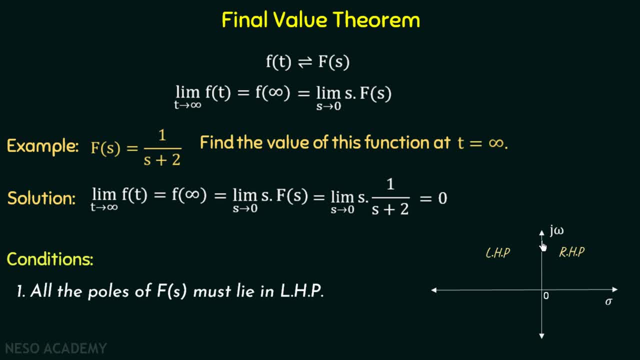 plane. When we draw the pole zero diagram in an s plane, then the part of s plane which is in the right half of origin is the right half plane and the part of s plane which is in the left half of origin is the left half plane. So for the final value theorem to be applicable, all the poles of 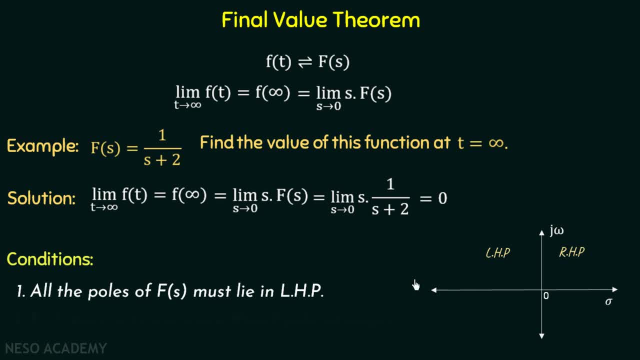 f? s must lie in the left half plane. Now condition number two is: f? of? s must not have more than one pole at the origin. f? s must not have more than one pole at the origin. So these are the two conditions which must be satisfied for the final value theorem to be. 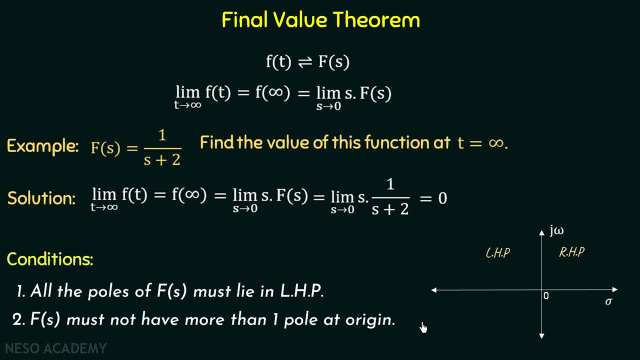 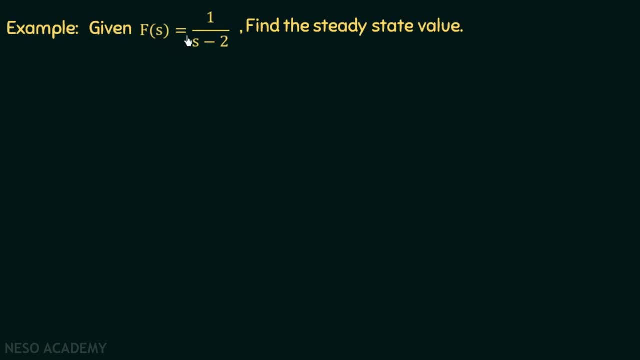 applicable. Now we will take some examples to understand that. if these two conditions are not satisfied, then why the final value theorem is not applicable. Given f of s equal to 1 over s minus 2, find the steady state value. So we are given a function, f of s equal to 1 over s minus 2 and we 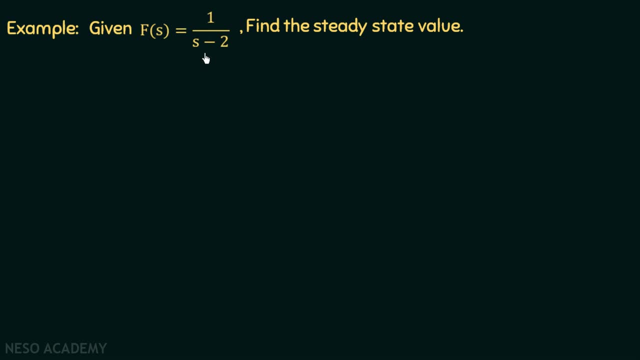 need to find out the steady state value or the final value of this function. So if we move on to the solution, we can see pole of f? s is at s equal to 2, which is in the right half plane. So 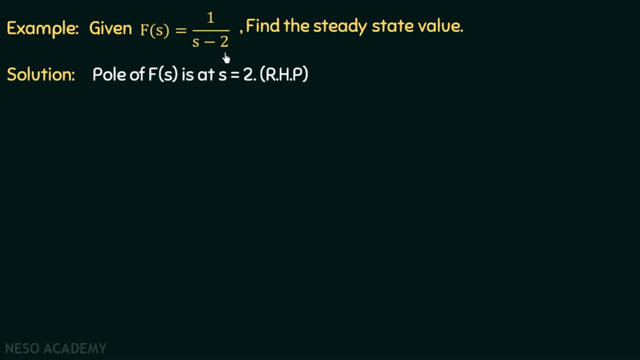 this function, f s is having a pole which is in the right half plane, So we can say final value theorem is not applicable. Now why it is not applicable? Let's check this by taking the inverse Laplace transform of this function. We will have f of t equal to e, power 2 t multiplied with u t. 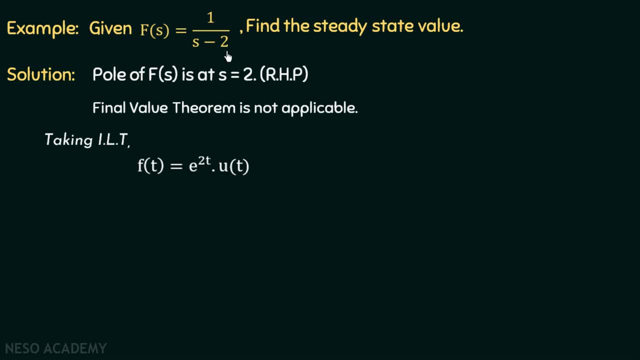 Inverse Laplace transform of 1 over s minus a is e to the power a t u t. That's why we are having f of t equal to e, power 2 t u t. This is an exponentially increasing function and if we plot this curve then it will be an exponentially increasing function. The final